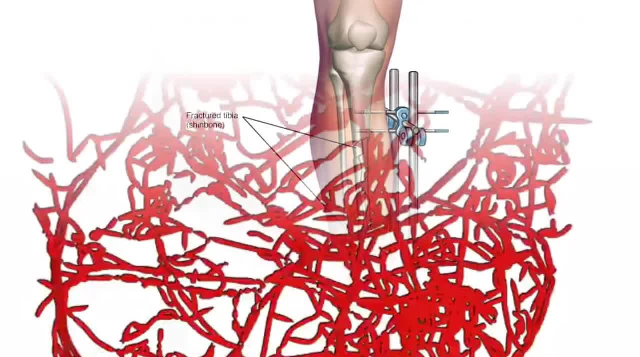 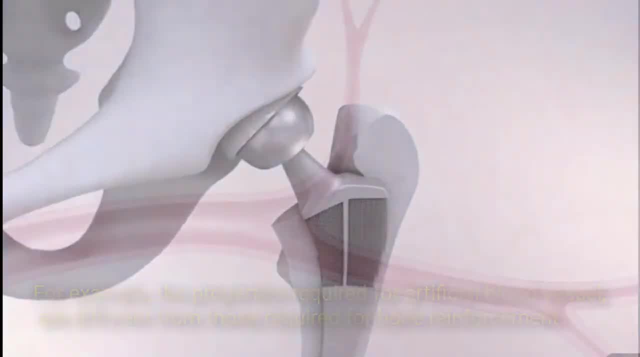 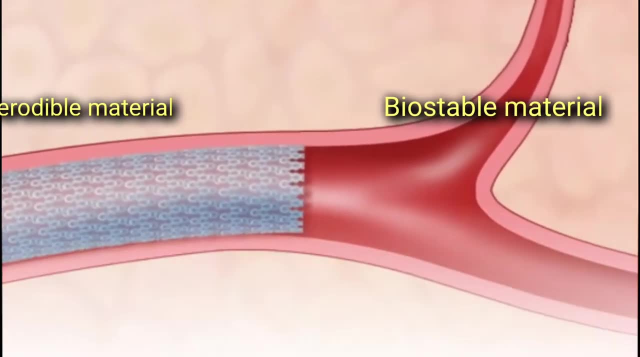 a different set of physical properties for each application. for example, the properties required for artificial blood vessel are different from those required for bone reinforcement. biomedical materials are grouped into two main categories: bioerodible material and biostable material. bioerodible materials: they are those materials that decompose to harmless product. 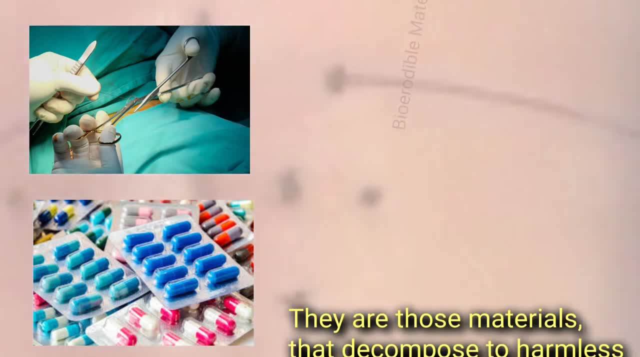 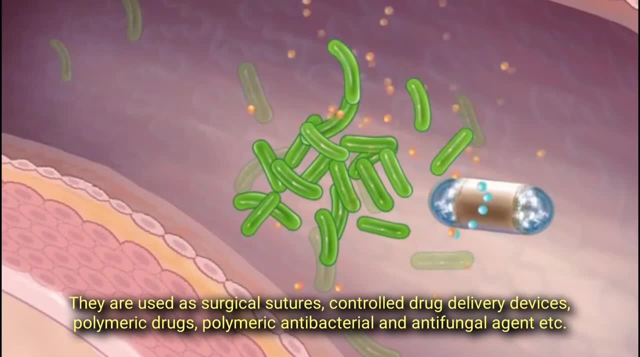 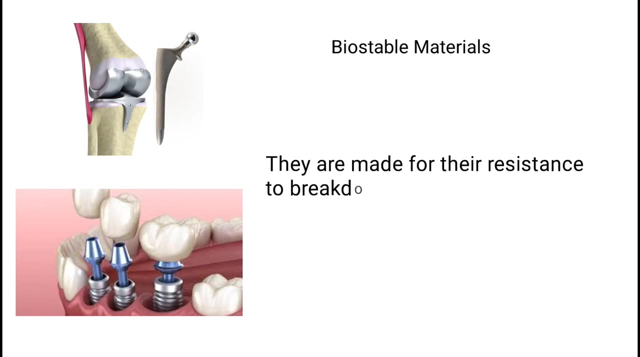 when implanted in the body, that is, they are unstable. they are used as surgical sutures, controlled drug delivery devices, polymeric drugs, polymeric antibacterial and antifungal agent, etc. biostable materials: they are made for their resistance to breakdown in a biological environment. they can be subdivided into. 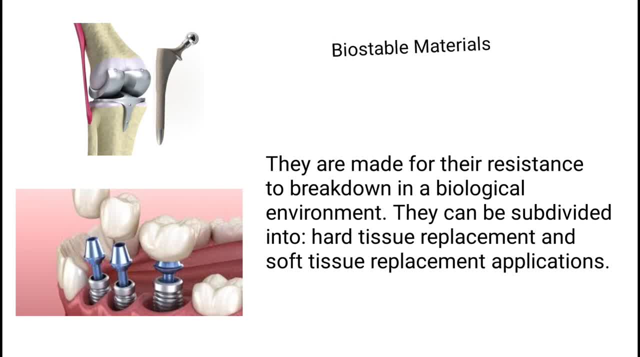 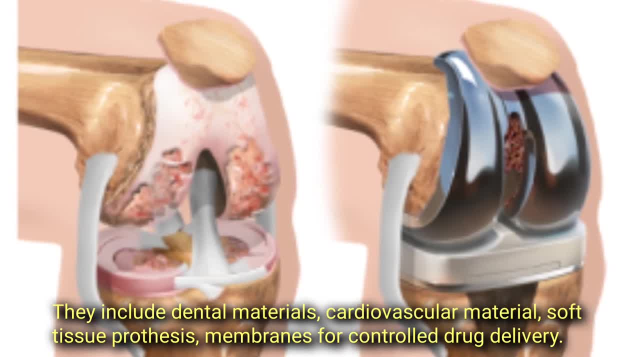 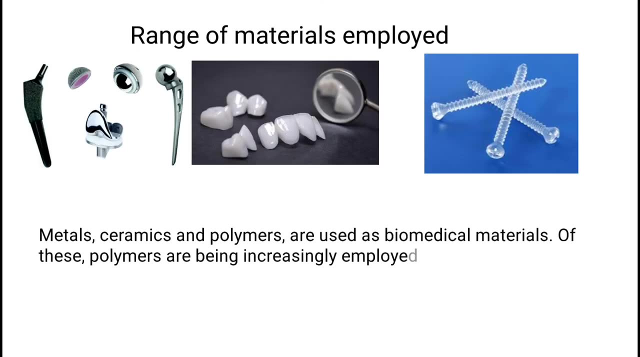 hard tissue replacements and soft tissue replacements applications. they include dental materials, cardiovascular material, soft tissue prosthesis, membranes for controlled drug delivery. range of material employed: metals, ceramics and polymers are used as biomedical materials. of these, polymers are being increasingly employed in medical devices, although metals and ceramics have important specialized. 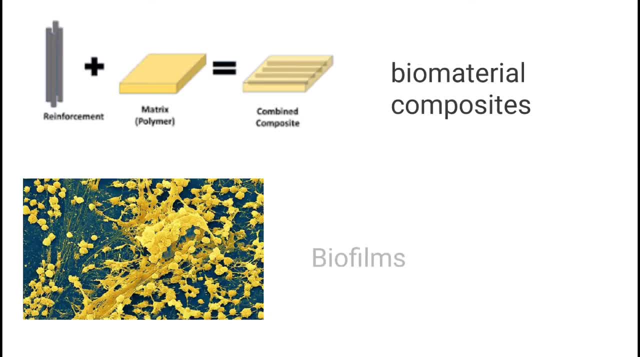 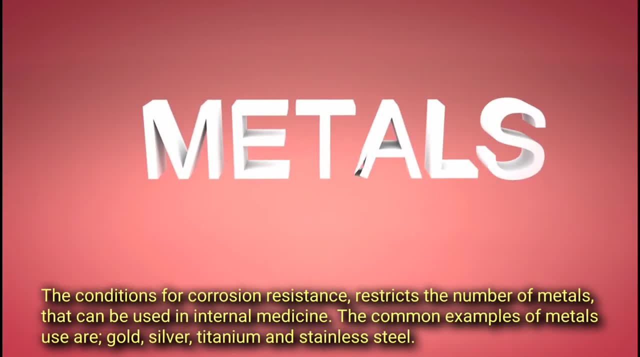 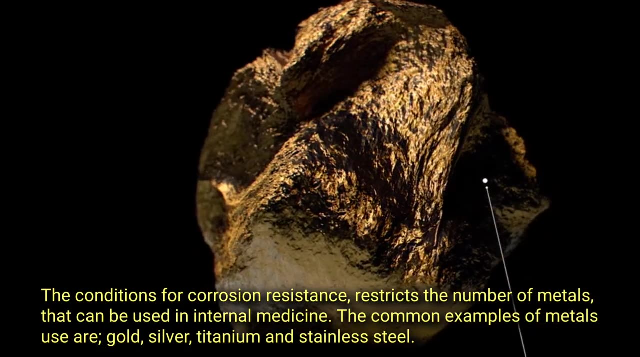 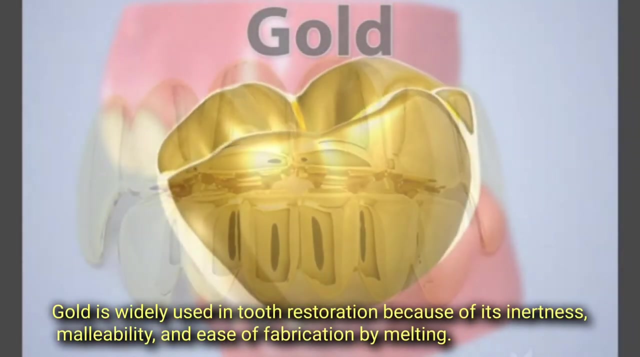 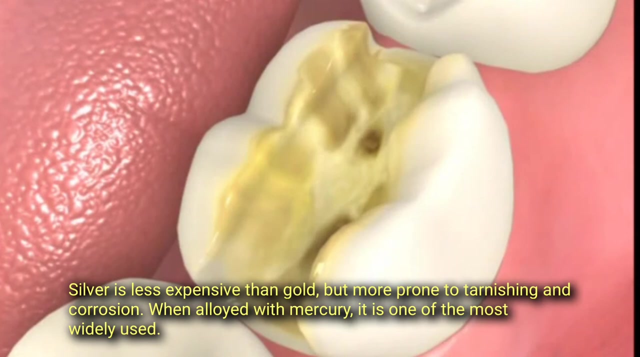 applications. other materials employed include biomaterials, composites and biofilms. metals: the condition for corrosion resistance. metal- 와 뭐 뇌메? Spotify in the sky. award for Hornet in the sky, provider of a very long time. we呀, or wäre ен. 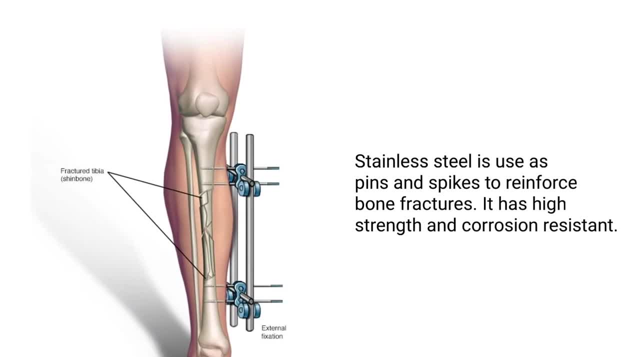 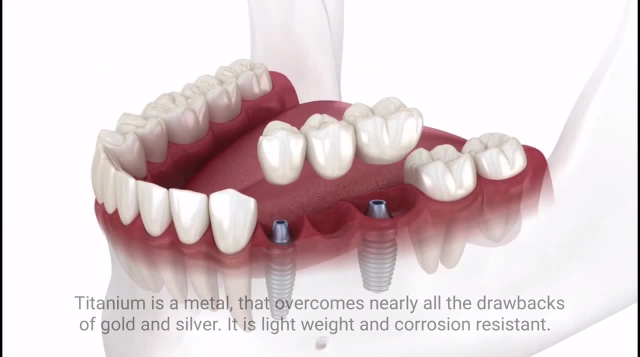 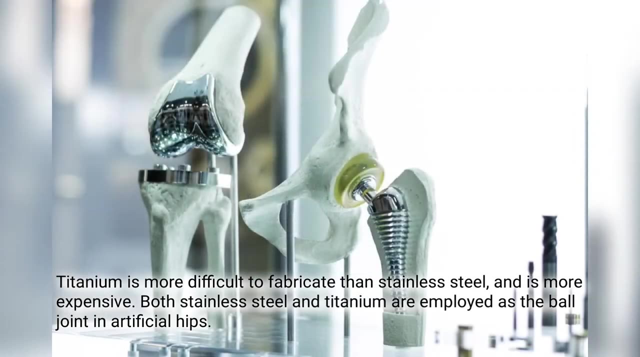 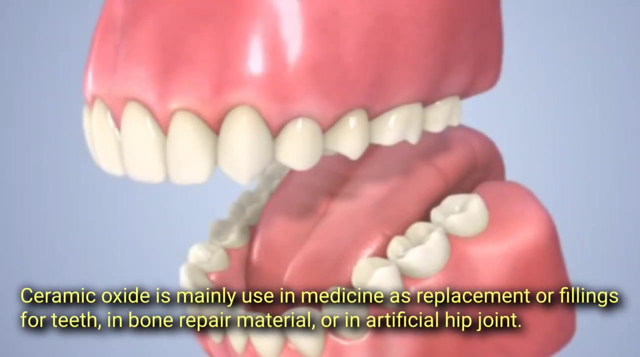 bone fractures. it has high strength and corrosion resistant. titanium is a metal that overcomes nearly all the drawbacks of gold and silver. it is lightweight and corrosion resistant. titanium is more difficult to fabricate than stainless steel and is more expensive. both stainless steel and titanium are employed as the ball joint in artificial hips ceramics. ceramic oxide is mainly. 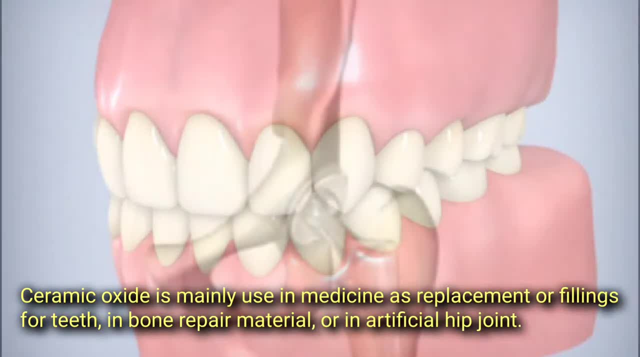 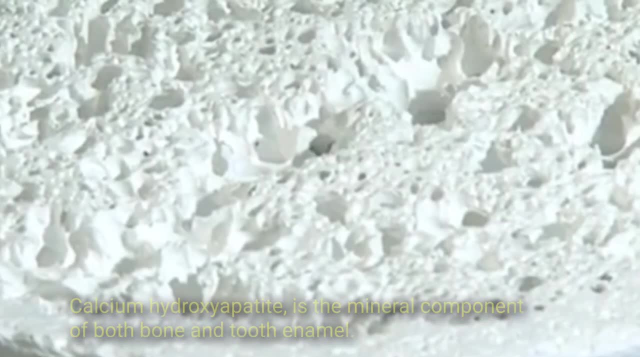 used in medicine as replacement or fillings for teeth, in bone repair material or in artificial hip joints. calcium hydroxyapatite is the mineral component of both bone and tooth enamel. various composites of calcium hydroxyapatite with polymers have wide use in dental restoration and bone. 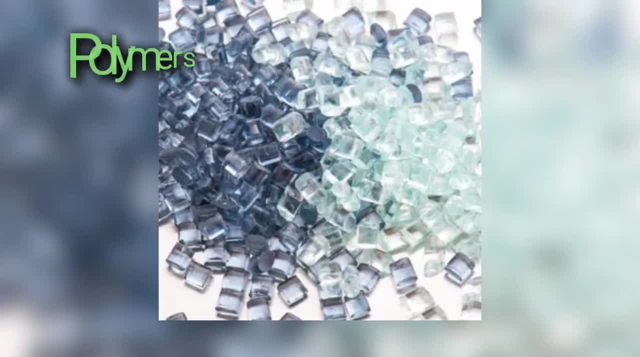 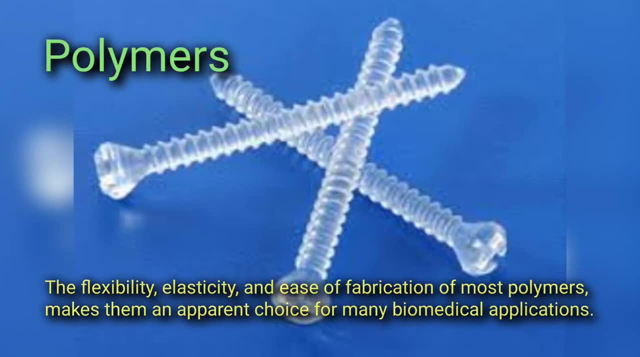 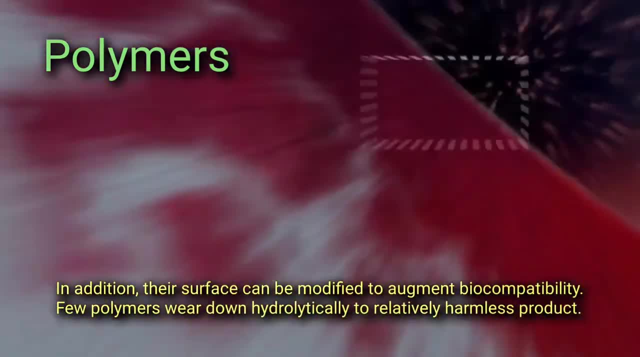 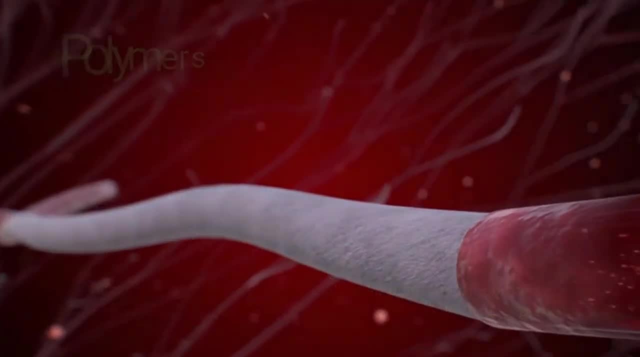 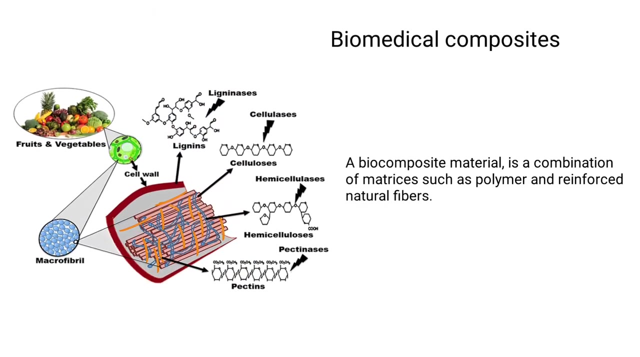 to bone. in addition, their surface can be modified to augment biocompatibility. few polymers wear down hydraulically to relatively harmless product. biomedical composites. a biocomposite material is a combination of matrices such as polymers and reinforced natural fibers. these composites imitates the morphology of 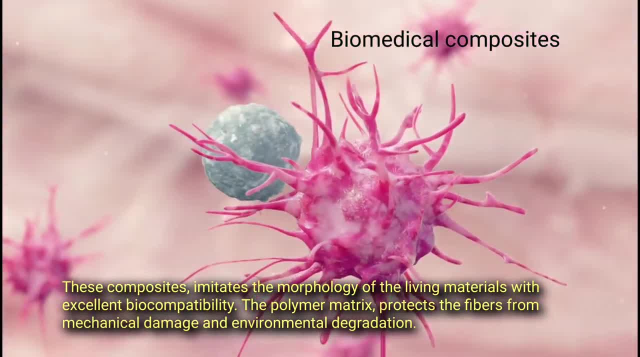 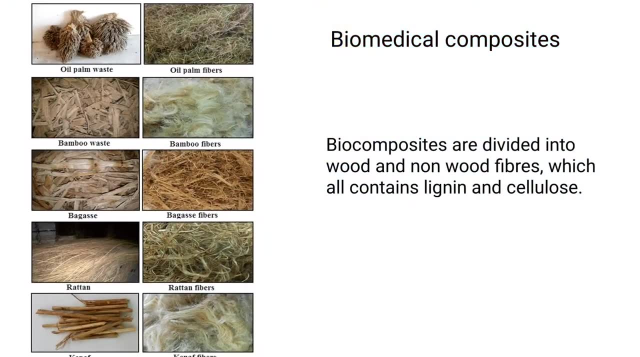 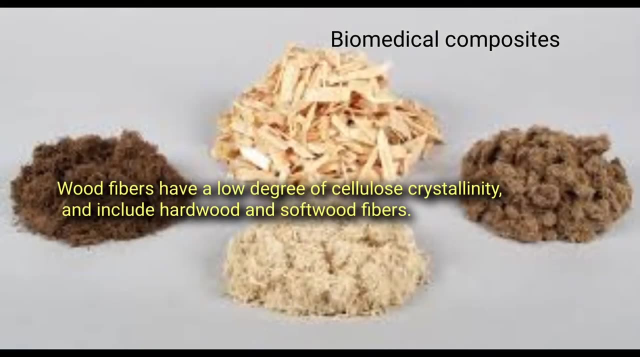 the living materials with excellent biocompatibility. the polymer matrix protects the fibers from mechanical damage and environmental degradation. biocomposites are divided into wood and non-wood fibers, which all contain lignin and cellulose. wood fibers have a low degree of cellulose crystallinity and include 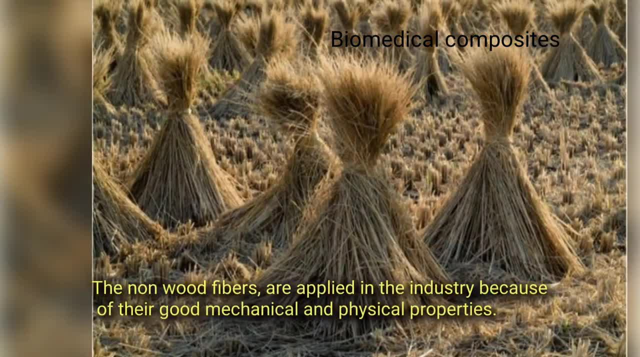 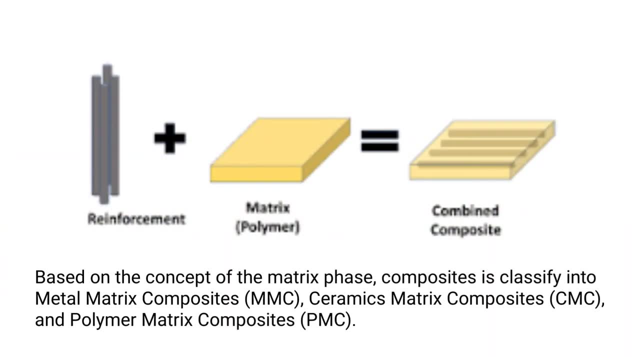 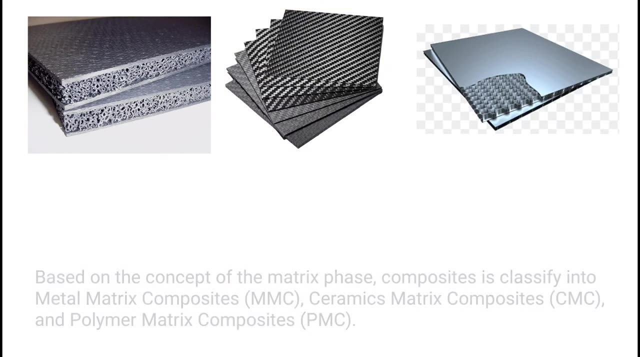 hardwood and softwood fibers. the non-wood fibers are applied in the industry because of the good mechanical and physical properties. based on the concept of matrix, phase composites is classified into metal matrix composites, ceramics matrix composites and polymer matrix composites, according to the basis of: 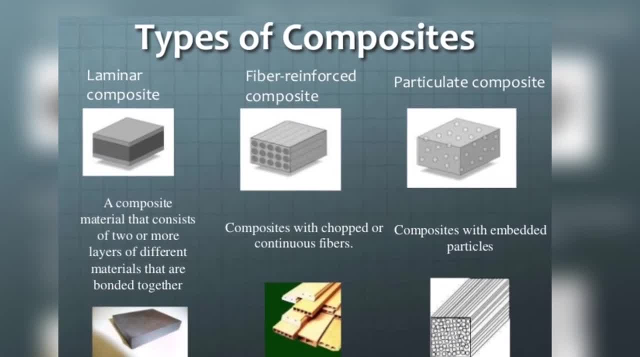 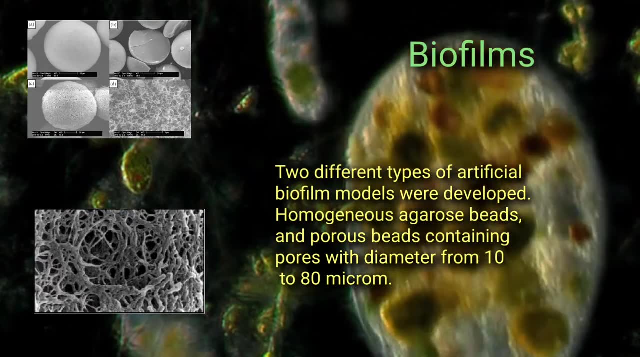 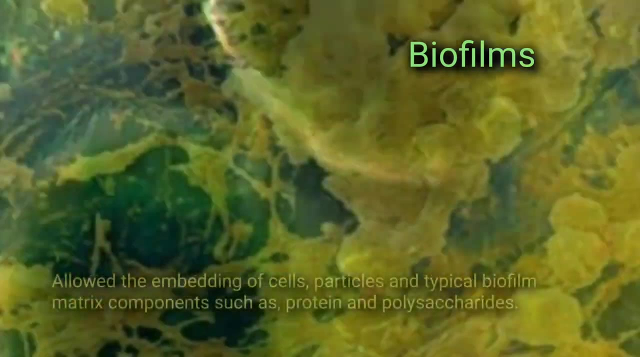 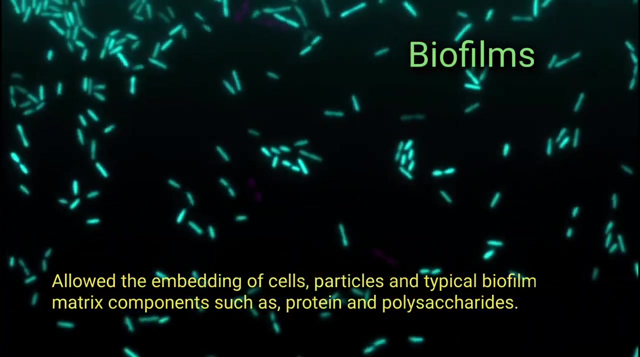 reinforcement. they are classified into fibrous, particulate and laminate composites biofilms. two different types of artificial biofilm models were developed: homogeneous agarose beads and porous beads containing pores with diameter from 10 to 80 micron allowed the embedding of cells, particles and typical biofilm matrix components such as proteins and polysaccharides. a brief. 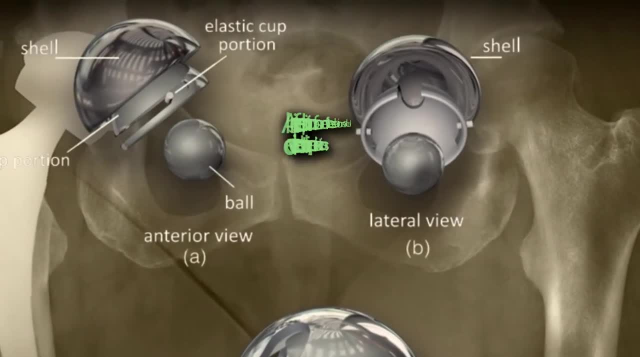 description of some of these biomedical device and their applications. a brief description of some of these biomedical device and their applications. a brief description of some of these biomedical device and their applications. one sutures- a surgical suture- is one of the most common medical devices used by. 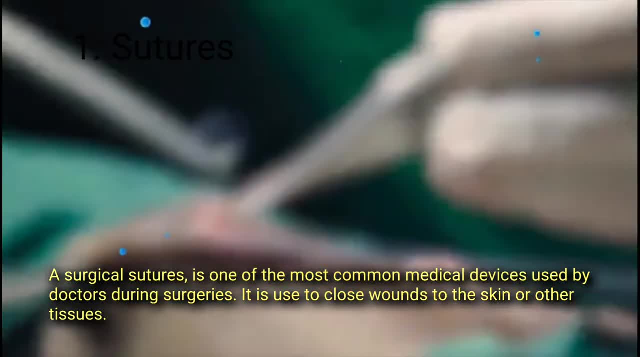 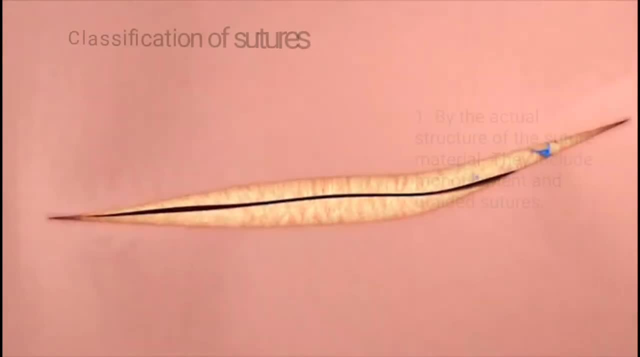 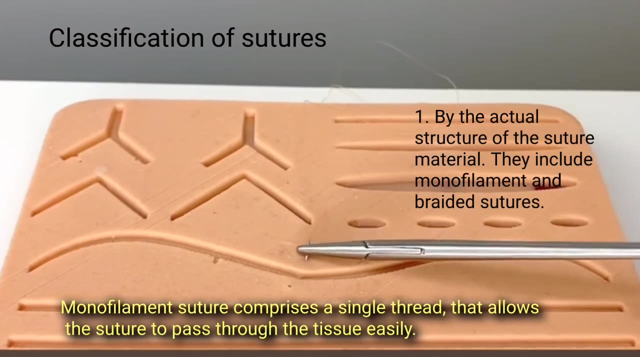 doctors. during surgeries, it is used to close wounds to the skin or other tissues. different types of sutures can be classified in many ways. firstly, by the actual structure of the suture material. they include monofilament and braided sutures. monofilament sutures comprises a single thread that allows 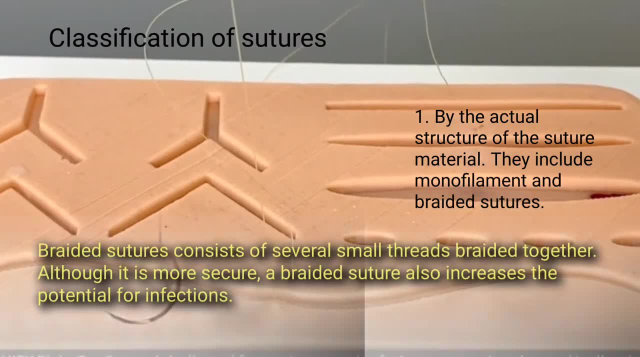 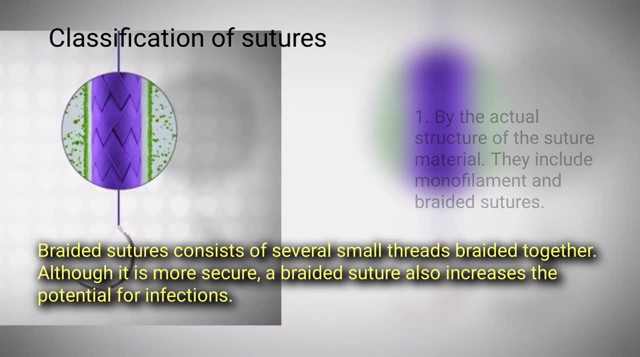 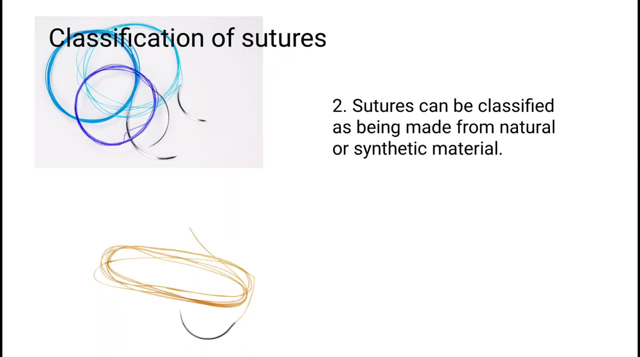 the sutures to pass through the tissue easily. braided sutures can assist of several small threads braided together. although it is more secure, a braided suture also increases the potential for infections. secondly, sutures can be classified as being made from natural or synthetic material. thirdly, by 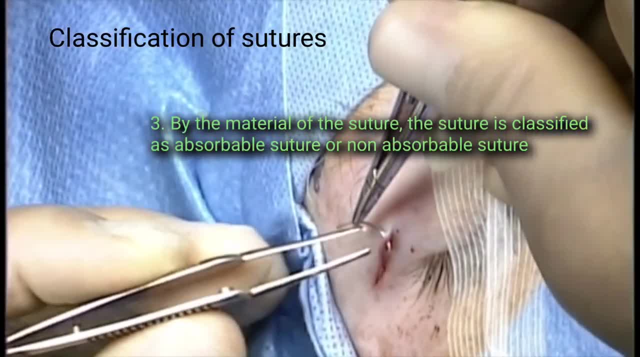 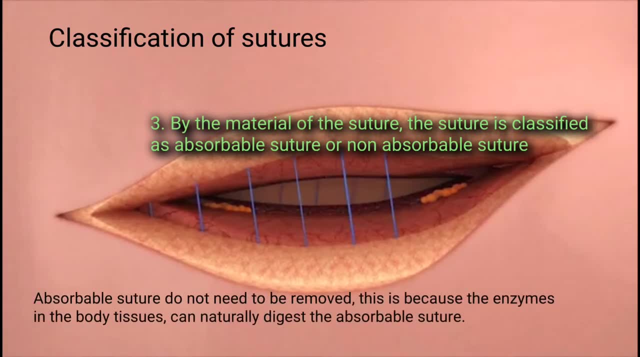 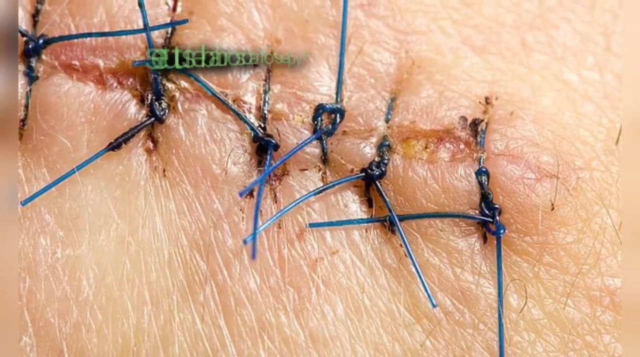 the material of the suture. the suture is classified as absorbable suture or non-absorbable sutures. absorbable sutures do not need to be removed. this is because the enzymes in the body tissues can naturally digest the absorbable suture. types of absorbable sutures: gut sutures, a gut. 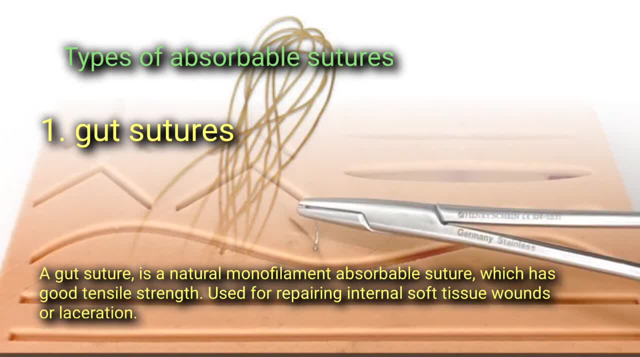 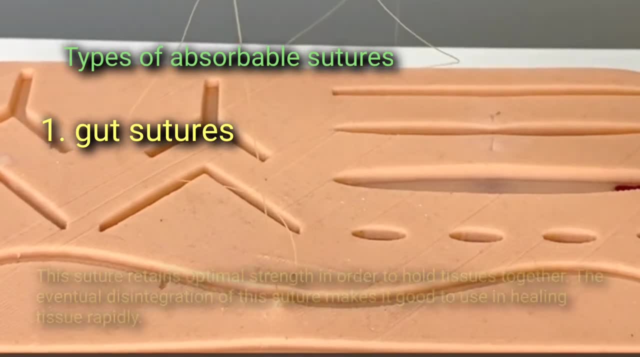 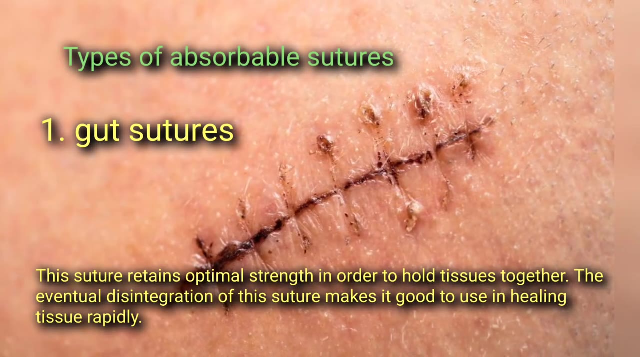 sutures is a natural monofilament absorbable suture which has good tensile strength, used for repairing internal soft tissue wounds or lacerations. this sutures retains optimal strength in order to hold tissue together. the eventual disintegration of this sutures makes it good to use in healing tissues. 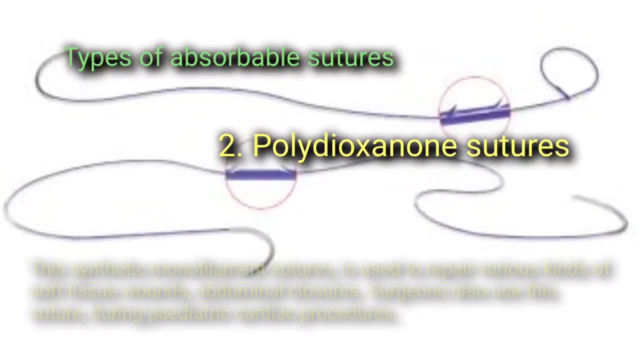 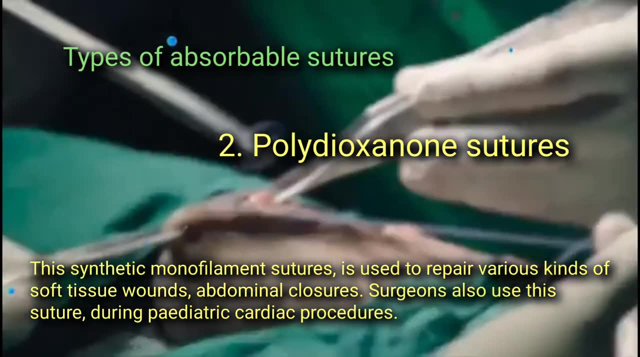 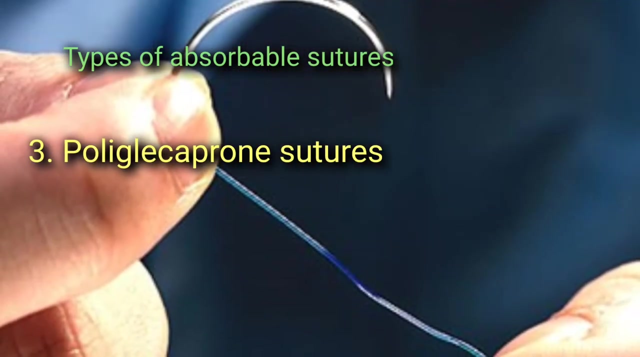 rapidly. poly dioxin own sutures. this synthetic monofilament sutures is used to repair various kinds of soft tissue wounds, abdominal closures. surgeons also use this sutures during pediatric cardiac procedures. polyglycaprone sutures: the polyglycaprone sutures is a synthetic 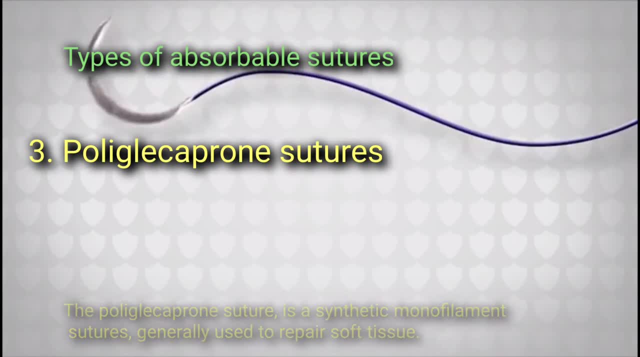 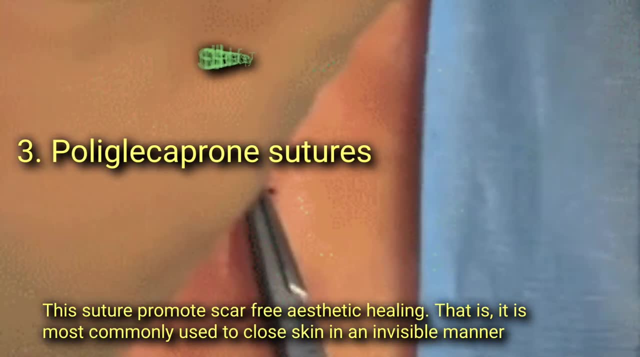 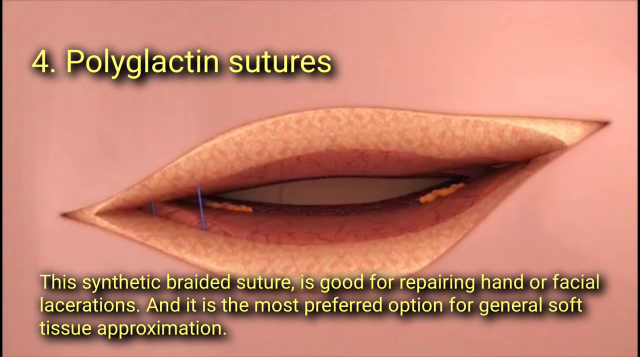 monofilament sutures generally used to repair soft tissue. this sutures promote scar-free aesthetic healing. that is, it is most commonly used to close skin in an invisible manner. polyglacton sutures- braided suture- is good for repairing hand or facial lacerations and it is the most preferred. 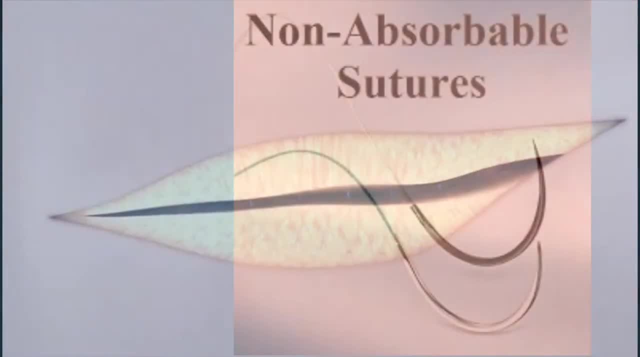 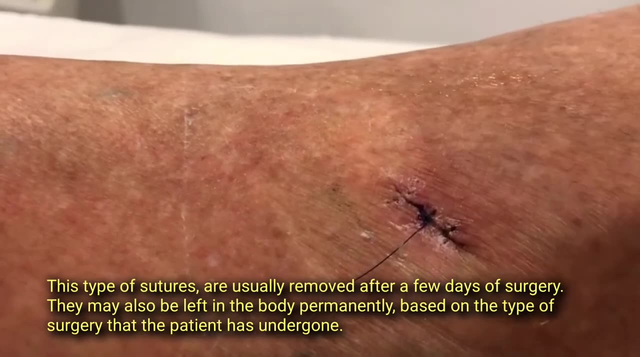 option for general soft tissue approximation non-absorbable suture. these types of sutures are usually removed after a few days of surgery. they may also be left in the body permanently, based on the type of surgery that the patient has undergone. this type of sutures are used. 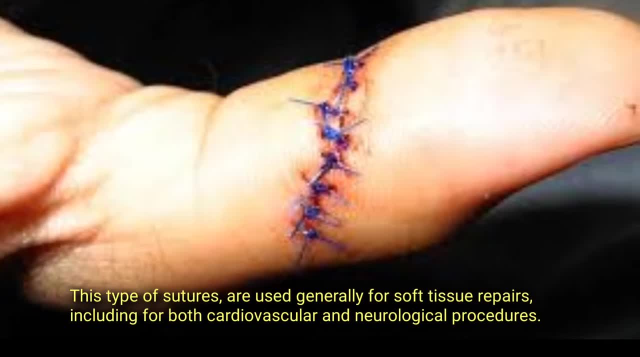 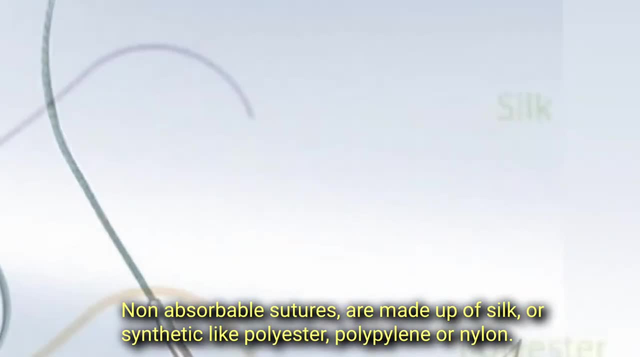 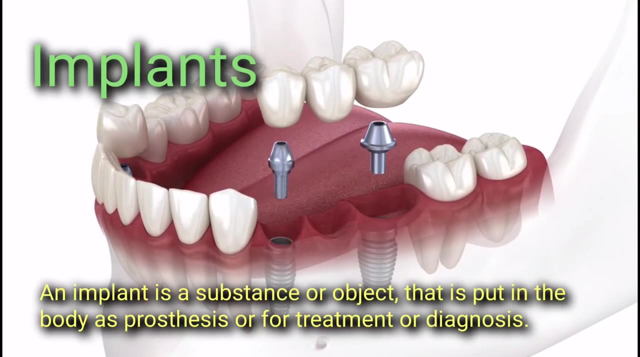 generally for soft tissue repairs, including for both cardiovascular and neurological procedures. non-absorbable sutures are made up of silk or synthetic, like polyester, polypillin or nylon implants. an implant is a substance or object that is put in the body as prosthesis or for treatment or diagnosis. many 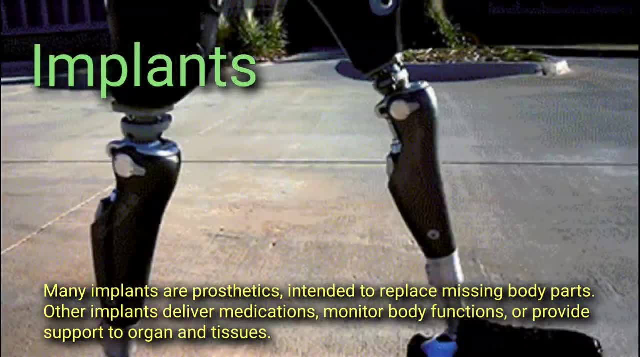 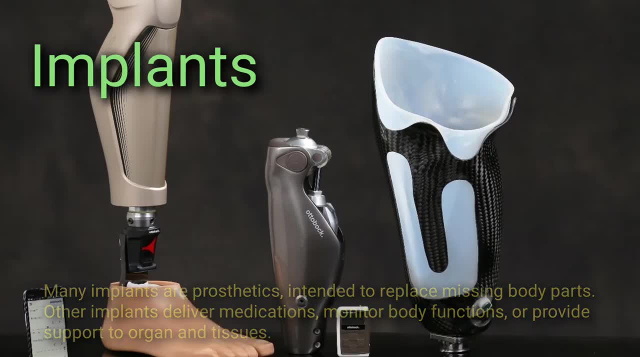 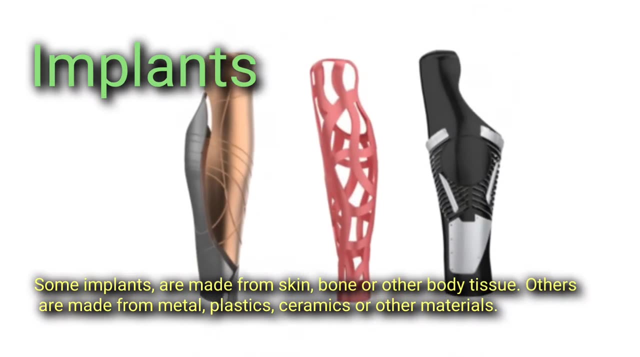 implants are prosthetics intended to replace missing body parts. other implants deliver medications, monitor body functions or provide support to organ and tissues. some implants are made from skin, bone or other body tissue. others are made from metal, plastics, ceramics or other materials. implants can be placed permanently or they can be removed. 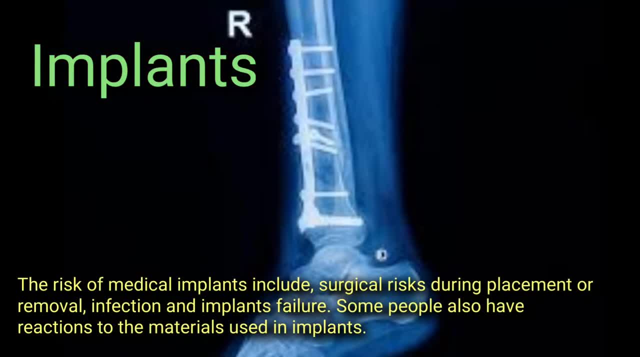 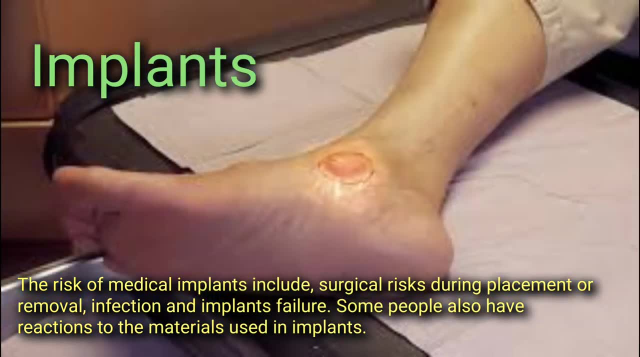 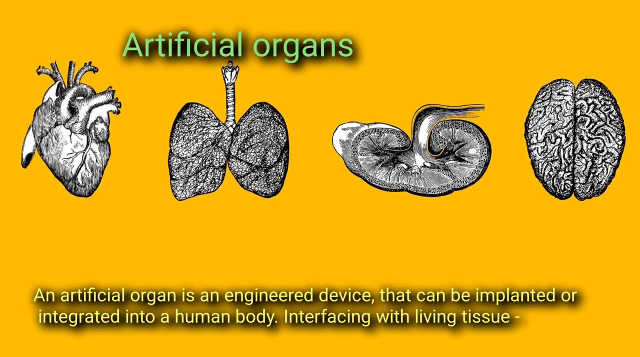 once they are no longer needed. the risk of medical implants include surgical risks during placement or removal, infection and implant failure. some people also have reactions to the materials used in implants. artificial organs: an artificial organ is an engineered device that can be implanted or integrated into a human body. 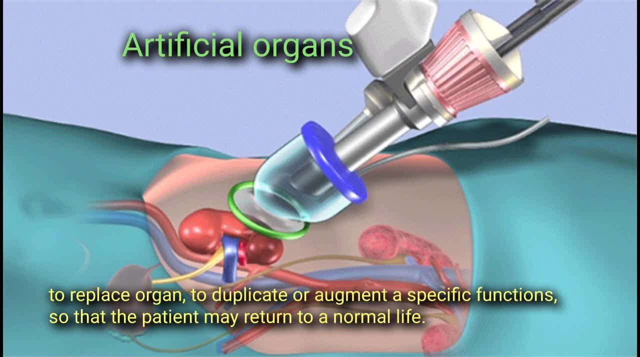 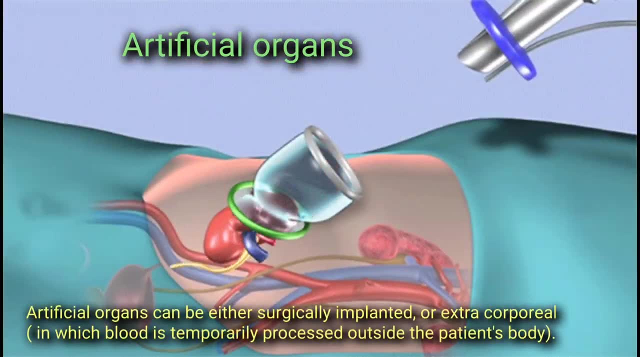 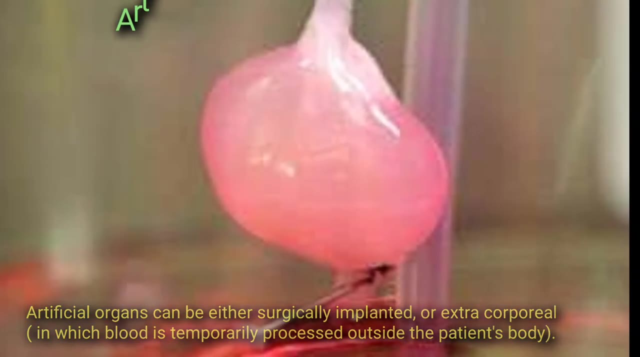 intero BLOOD tissue to replace organ, to duplicate or augment a specific functions so that the patient may return to a normal life. Artificial organs can be either surgically implanted or extra-corporeal, in which blood is temporarily processed outside the patient's body. 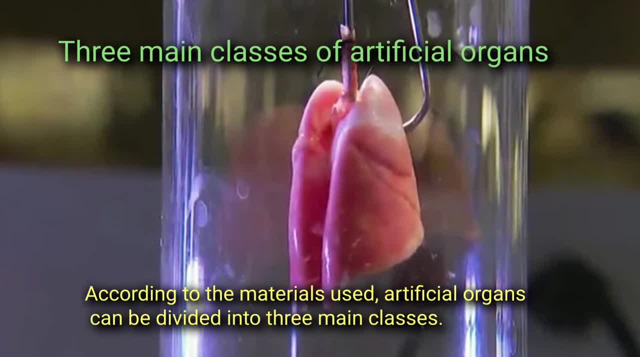 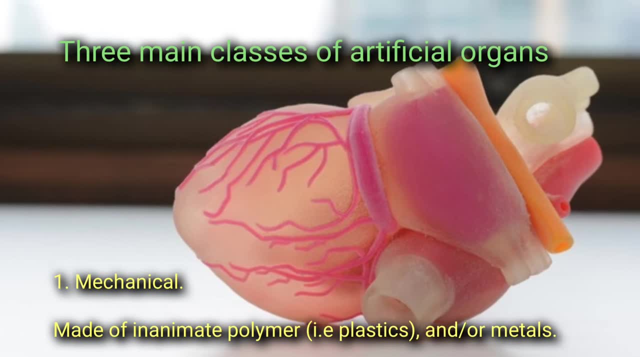 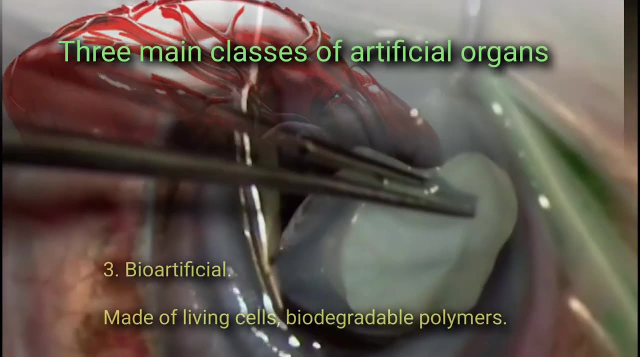 According to the material used, artificial organs can be divided into three main classes: 1. Mechanical, made of inanimate polymer, ie plastics and or metals. 2. Mechanical made of partially living cells and inanimate polymer and or metals. 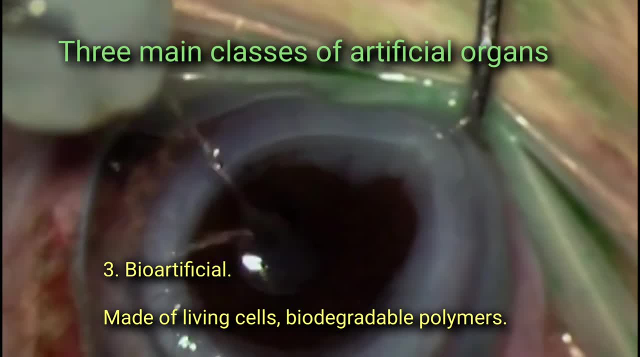 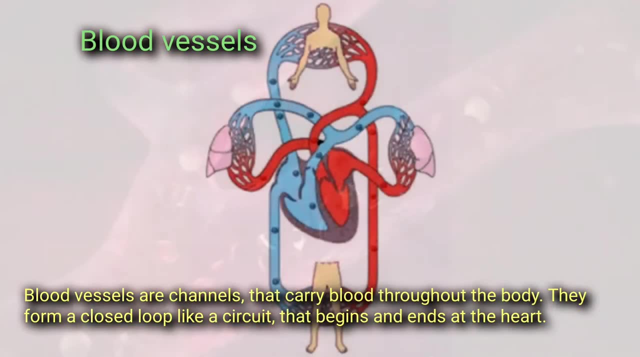 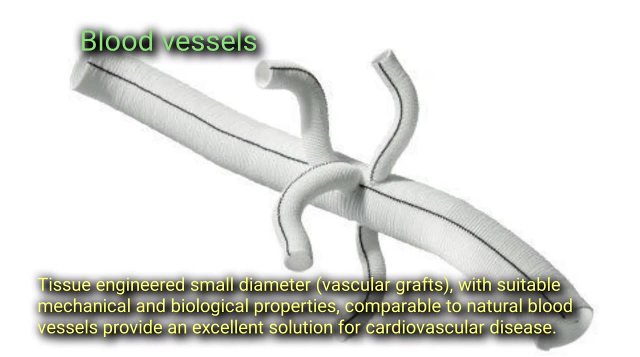 3. Bioartificial: made of living cells, biodegradable polymers. Blood vessel. Blood vessels are channels that carry blood throughout the body. They form a closed loop like a circuit that begins and ends at the heart Tissue. engineered small diameter vascular grafts with suitable mechanical and biological 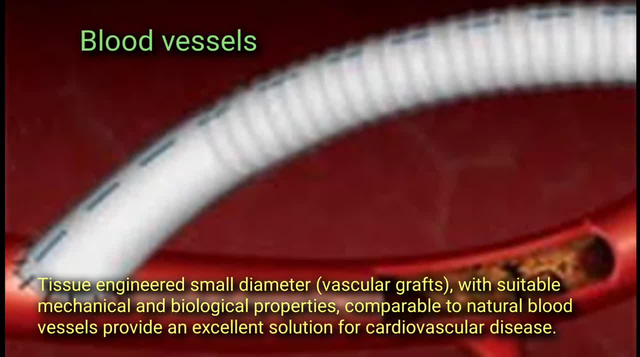 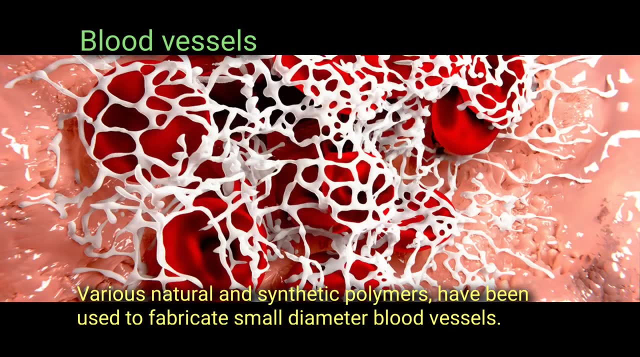 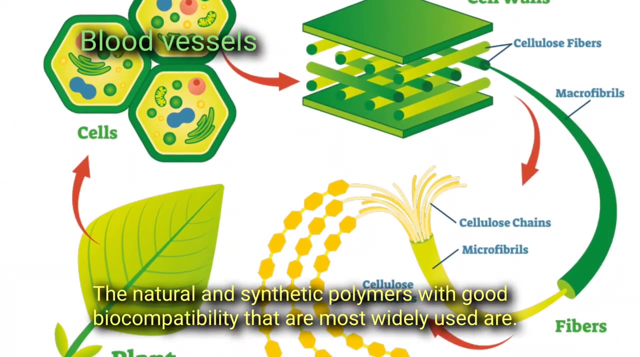 properties comparable to natural blood vessels provides an excellent solution for cardiovascular disease. Various natural and synthetic polymers have been used to fabricate small diameter blood vessels. The natural and synthetic polymers with good biocompatibility that are most widely used are: 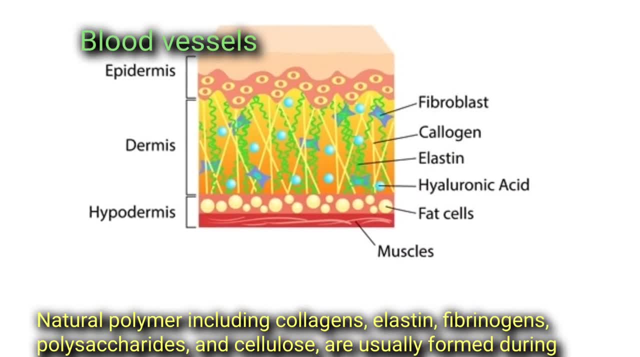 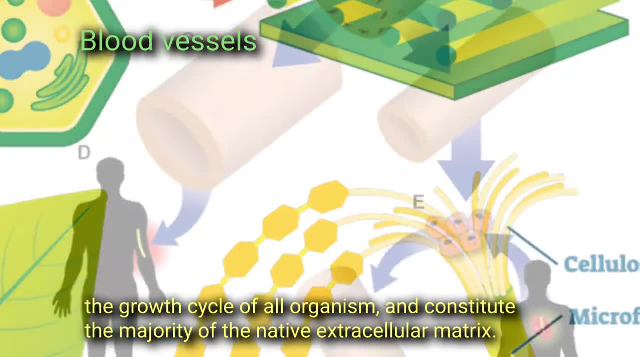 Natural polymers, including collagens, elastin, fibrinogens, polysaccharides and cellulose, are usually formed during the growth cycles of all organism and constitute the majority of the native extracellular matrix. 3. Biocompatibility: